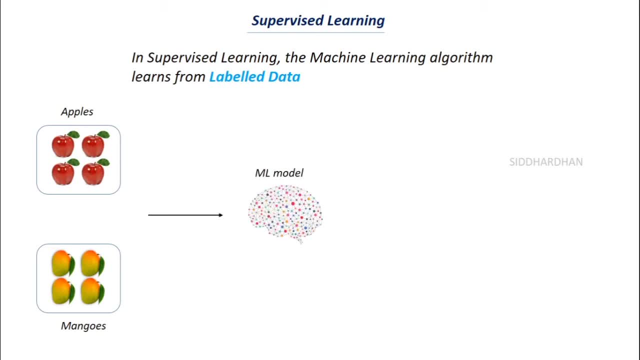 OK, and we feed these images to our ML model. and what it does? it tries to Find the relationship between these images and it maps it to the label, which is apples and mangoes. OK, now it knows, you know how an apple looks and how a mango looks. 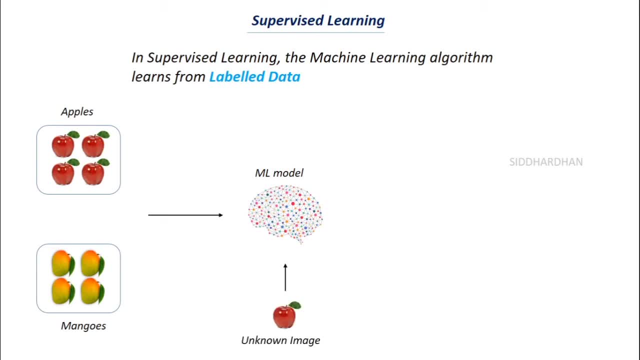 OK. so once it learned from the data, when you give an unknown image, it can predict correctly whether it is an apple or a mango. So this is how supervised learning works. So the important point to note here is we are training the machine learning model with data which is labelled. 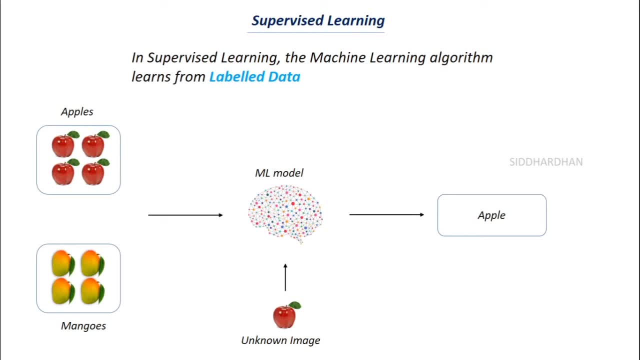 OK. so in case of unsupervised learning, we don't give the machine learning model a label. OK, so in case of unsupervised learning, we don't give the machine learning model a label. OK, so in case of unsupervised learning, we don't give the machine learning algorithm the labels. 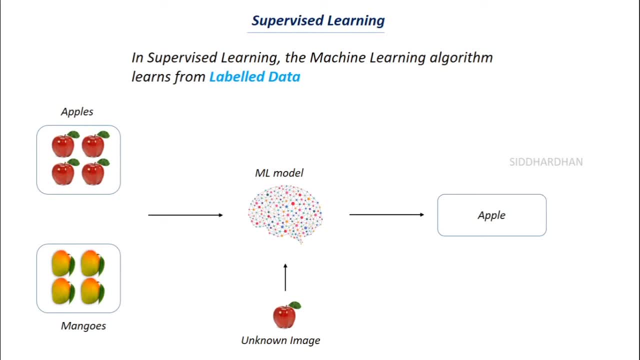 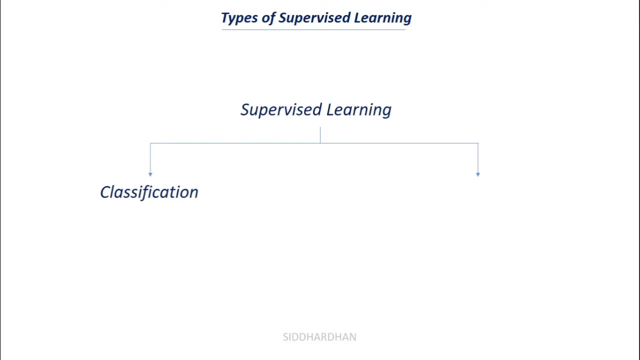 OK, so that is the difference between supervised and unsupervised learning. OK, now let's discuss about the types of supervised learning. There are two main types of supervised learning. One is classification and another one is regression. OK, so what is meant by this classification and regression? 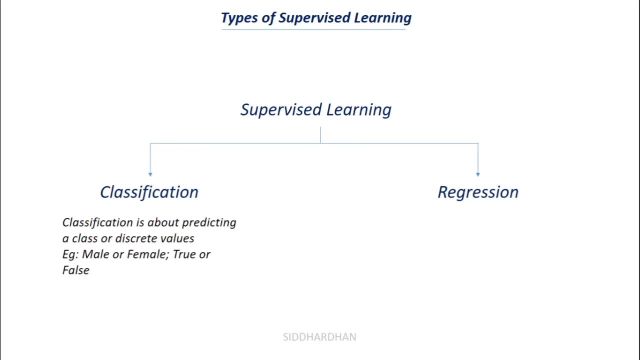 So classification is about predicting a class or discrete value. OK, so that is just these class or labels. OK, so there is not continuous values like numbers, So it will predict. you know the problem statement: we have to predict whether it's a male or female, true or false. 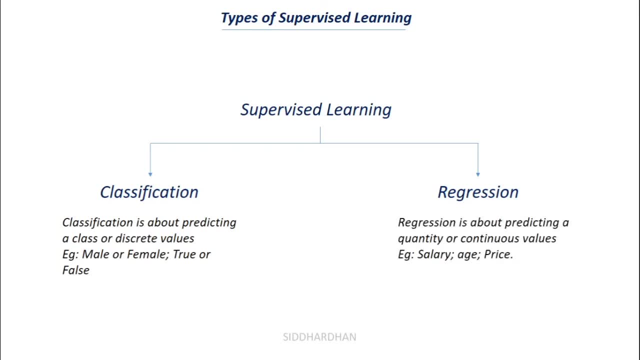 like that. okay, so there will only be classes and in regression we try to predict a continuous values, for example, like the salary, age and price. okay, say for example: um, we need to predict salary of a person from his work experience. okay, so the salary will be in a continuous number, right? 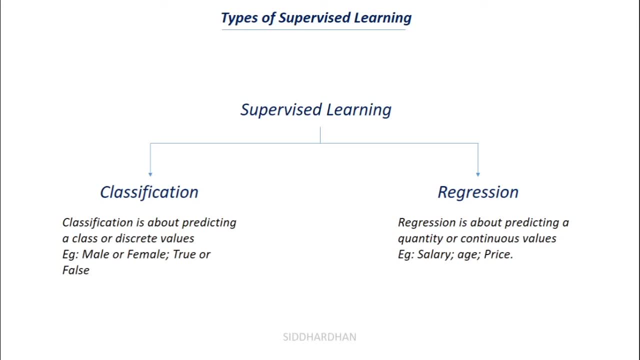 so those kinds of problem statements are done using regression models. okay, in classification we just predict it's, you know, whether true or false, or male or female. say, for example, the example we have seen before where our model classifies the images into apples or mangoes, whereas in regression we find a particular number. okay, so let's try to understand this with another. 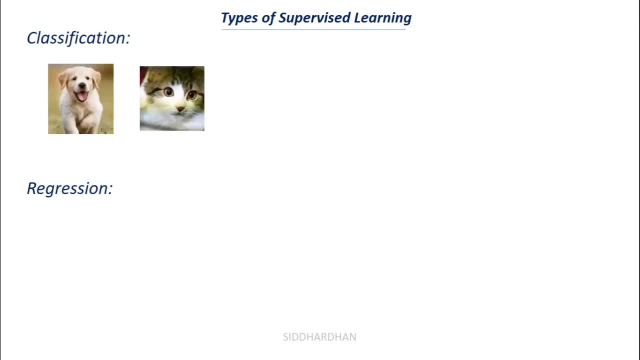 example. so first of all, classification. so we want our machine learning model to see an image and recognize whether the image is, you know, a dog or cat. so what we will do is we will give the labels and the data to our machine learning model so it maps with that label and the images. now we can. 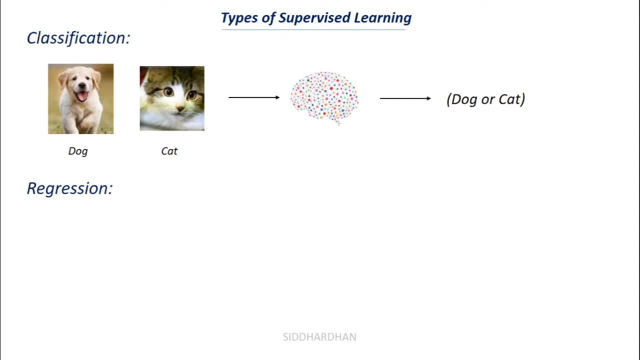 tell whether it is a dog or cat. so this represents classification, because we are just classifying the image into either dog or cat. okay, so there is no middle values, right? so there is not any decimal values here, it is just binary in this case. now let's discuss about an example for regression. 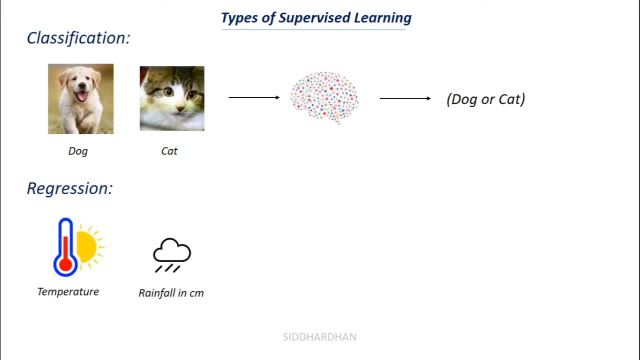 let's say that we need to predict the rainfall in centimeter value for a given temperature or pressure and different factors on which the rainfall depends. okay, so what we will do is we will train our machine learning model with this data, like, for example, so we will tell the machine 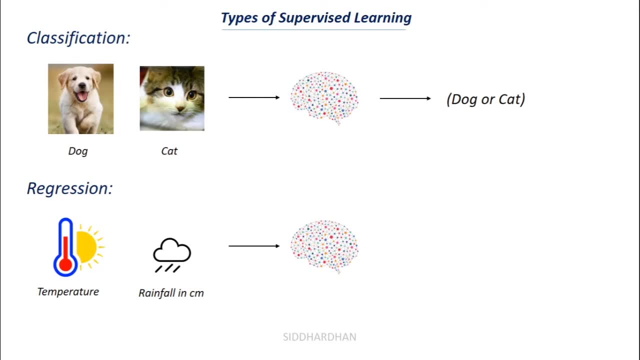 learning model that for this temperature there will be this much amount of rainfall, and for you know different cases like this, and when the model is learned from the data, when we give a new temperature value, it can tell you how much rainfall we can expect. so the rainfall in centimeter will. 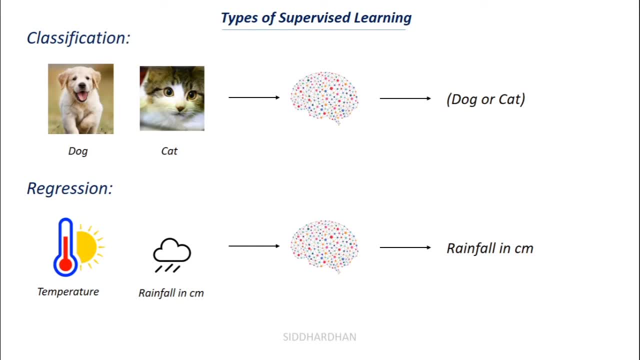 be a continuous value, it can be a decimal value, right? so this is called as regression. so this is called as regression, and this is called as regression, and this is called as classification. so in classification we try to, you know, predict the class or type, but in regression, 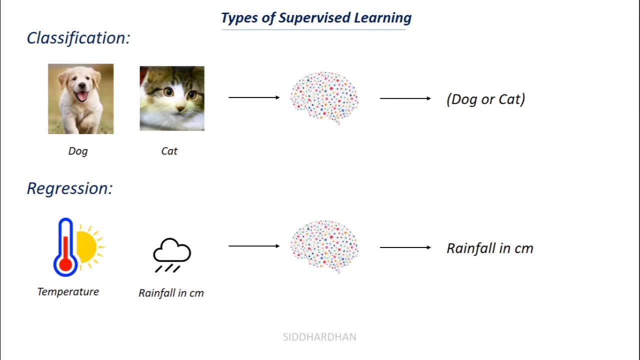 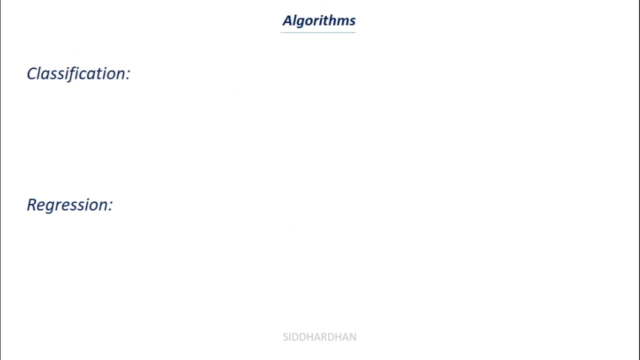 we try to predict or we try to find a number. okay, so that is the difference between classification and regression. so there are various, lot of different types of application on classification and regression, so which we will see in our later videos, in our project videos. okay, now let's see. 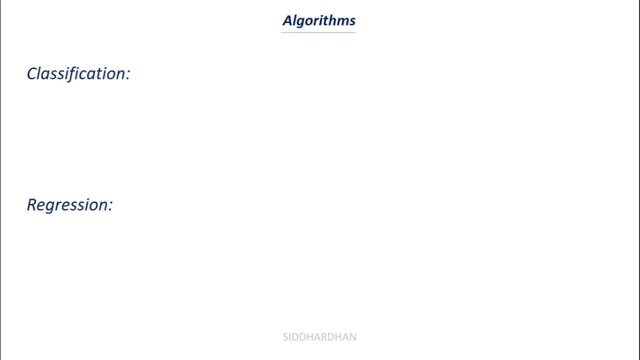 what are some most important algorithms for classification and regression? decision tree classification, random forest classification, k nearest neighbor classification. so these are some examples of classification algorithms and regression model. algorithms includes logistic regression, polynomial regression and support vector machine regression. so it's okay if you don't understand what is meant. 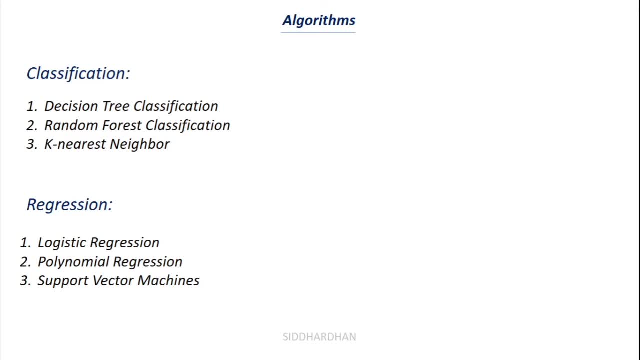 by these algorithms. so we will be working on each type of algorithms once we start doing the hands-on part, so i'll be explaining about them in more detail once we start those videos. okay, so that's it for this video. in the next video, let's discuss about what are the most important. 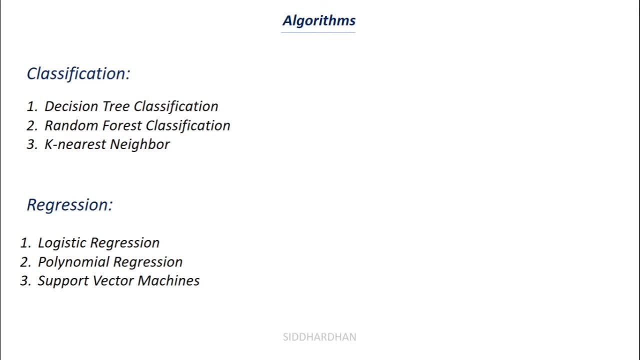 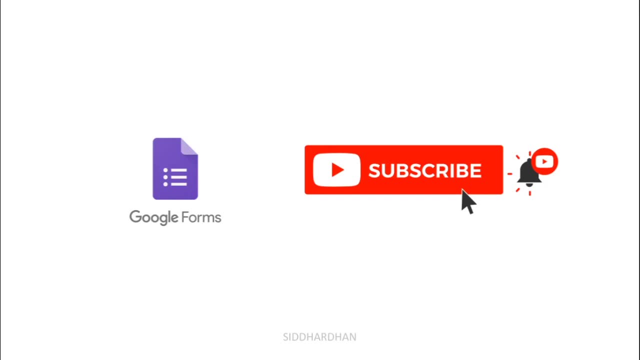 algorithms for classification, what is unsupervised learning and what are its types, as we did in this video? okay, so that's it from my side. do check out the google forms link in the description and try to answer those questions. so, if you liked the video, if you enjoy the video, do subscribe and